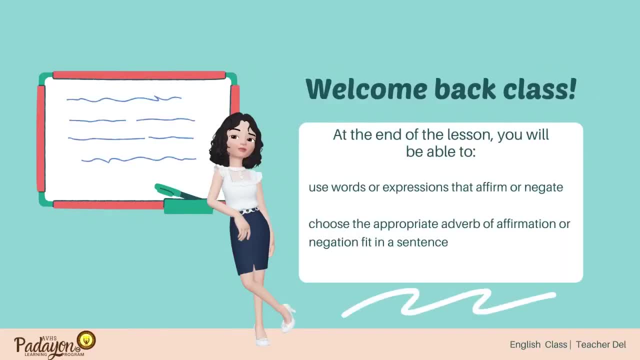 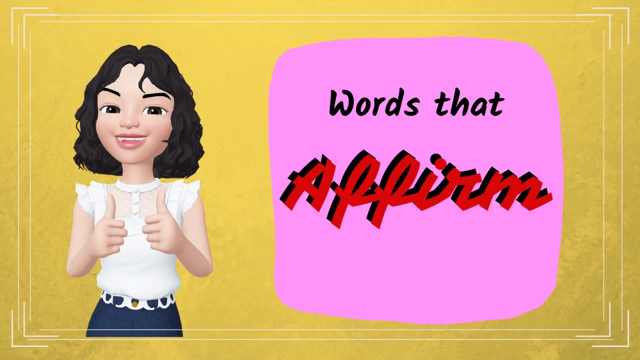 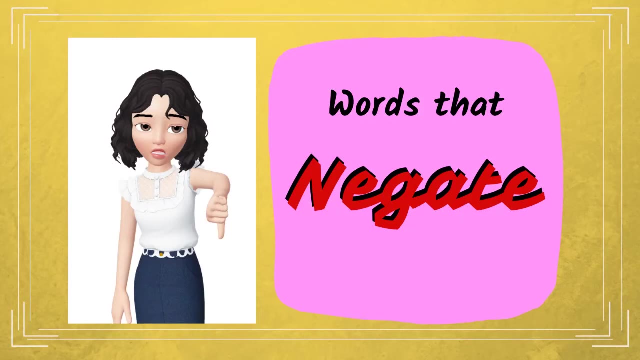 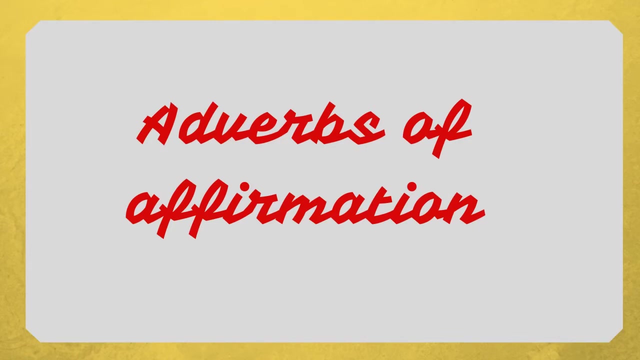 Hello everyone, In this video you will be learning about words that affirm and words that negate. So first let's go to words that affirm or adverbs of affirmation. Adverbs of affirmation are used to denote certainty or emphasize action. So affirm: you, agree to something. 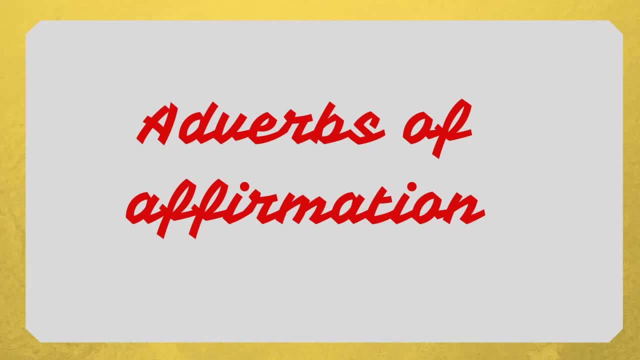 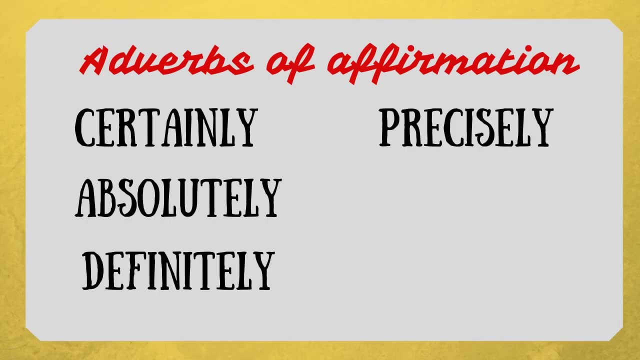 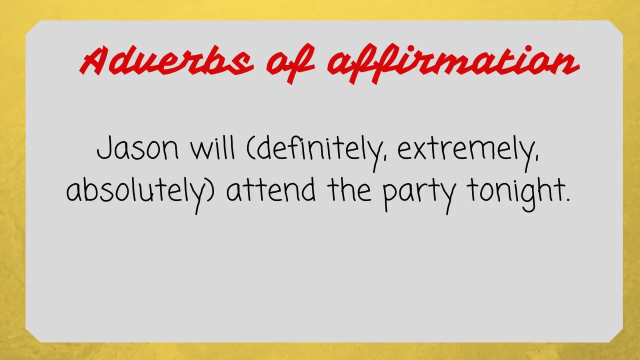 So examples of adverbs of affirmation are Certainly, Absolutely, Definitely, Precisely, Positively and Surely. Now, these are just some of the adverbs of affirmation. There's a lot more out there. Okay, so let's take a look at this sentence. 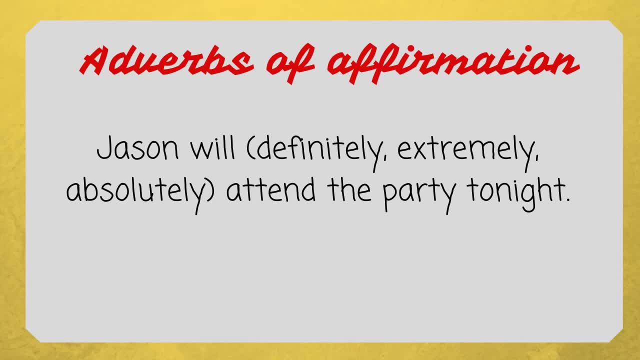 The adverb of affirmation that is not really appropriate for the given sentence. Again, we will be choosing the adverb of affirmation that is not appropriate to complete the sentence. Okay, so Jason will definitely, extremely, absolutely, attend the party tonight. 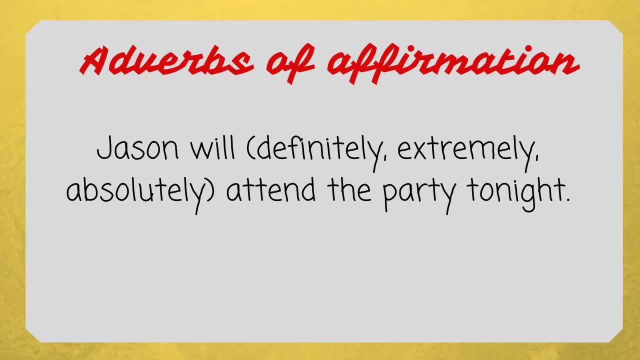 So what is the adverb of affirmation that is not that appropriate for this sentence? The answer is: Extremely. Extremely is a bit far-fetched or a bit, you know, not really that appropriate. Extremely is a bit far-fetched or a bit, you know, not really that appropriate in this sentence. 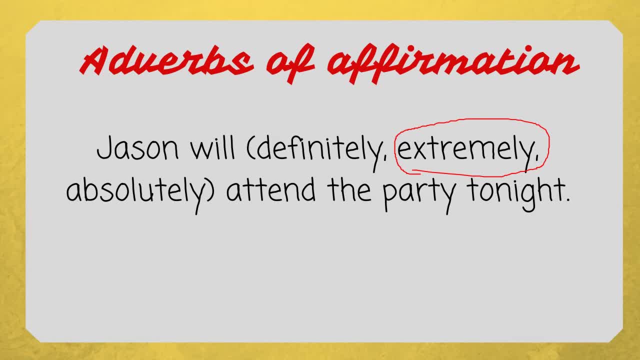 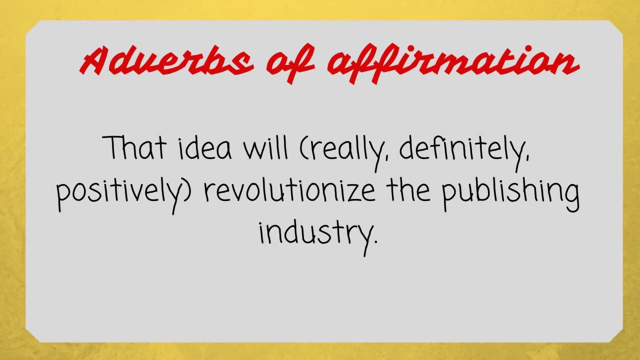 When we choose the word definitely, it fits just right in the sentence: Jason will definitely attend a party tonight, or will absolutely attend a party tonight, And extremely is a bit too much already. Now let's go to the next one. The idea will really definitely, or positively, revolutionize the publishing industry. 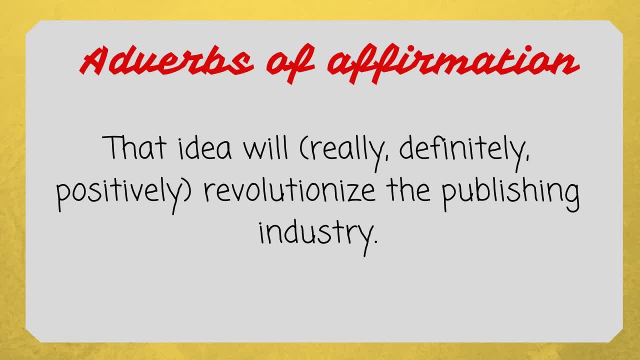 So what's the adverb of affirmation that is not really appropriate for this sentence. It is Positively Okay. The idea will really revolutionize the publishing industry, or will definitely revolutionize the publishing industry. So this sentence is trying to give us an idea that there's that certainty. 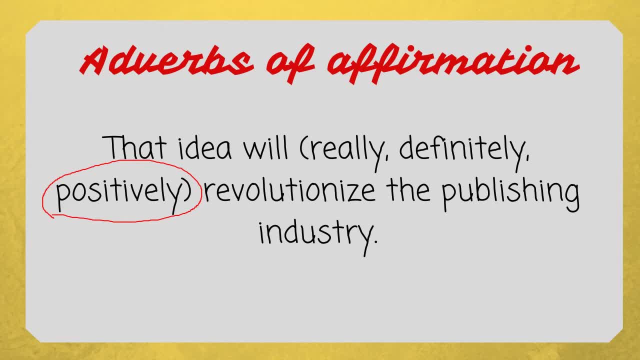 That certainty, That it's really sure, Sure na sure, Really definitely na. But when we say positively, positive, So it's just positive, Positive, lang There's. It's like it's far from being sure, Though it's positive. 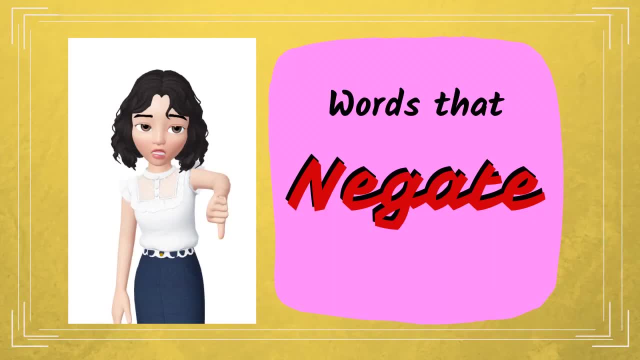 Okay, If you know what I mean, Now we will proceed to words that negate. Now, when we say negate or there's a negation, it means to turn something down, or to deny, or to disagree or to disapprove an action. 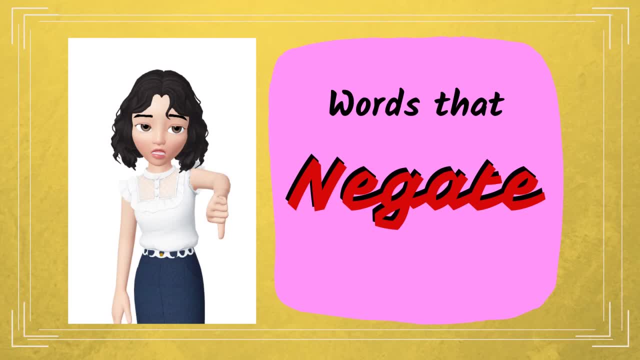 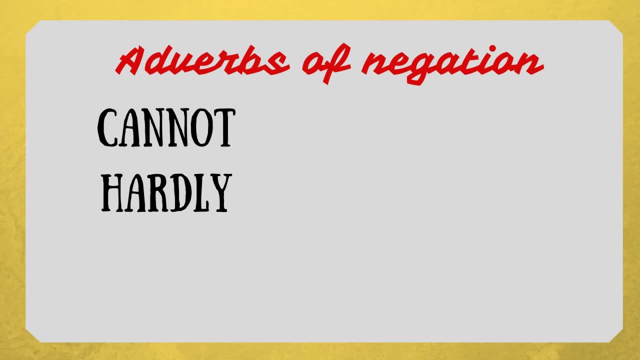 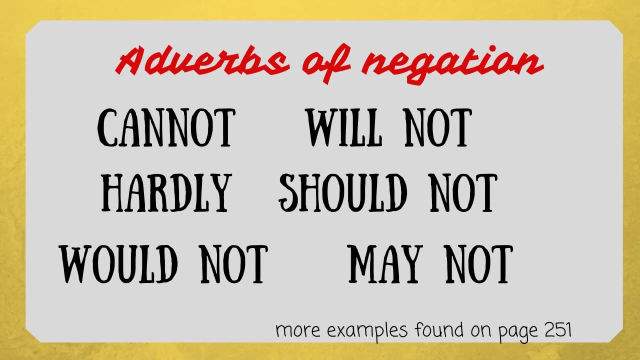 Now we will have here adverbs of negation. Now what are those We have? cannot, hardly, would not, will not, should not, may not, and there's a lot more examples that you can find in page 251.. 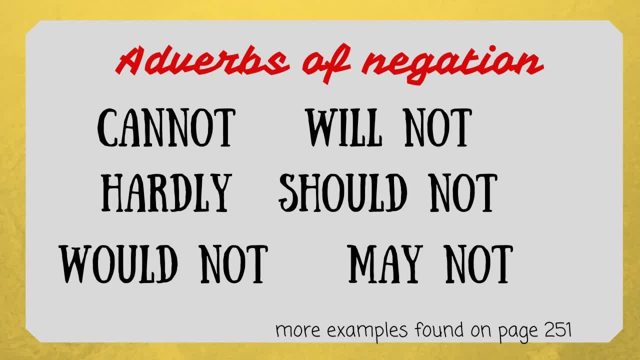 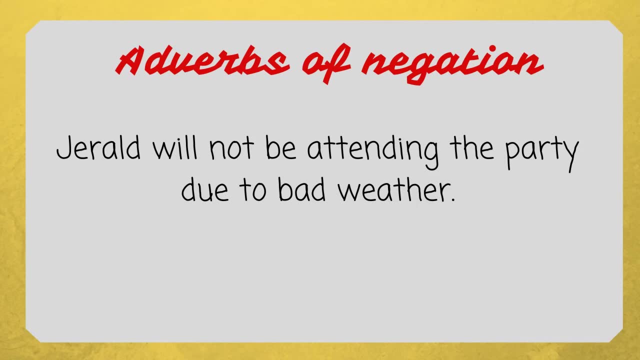 In page 251 of your book. So Now let's take a look at adverbs of negation used in a sentence. Gerald will not be attending the party due to bad weather. Now the adverb of negation used in this sentence is: will not. 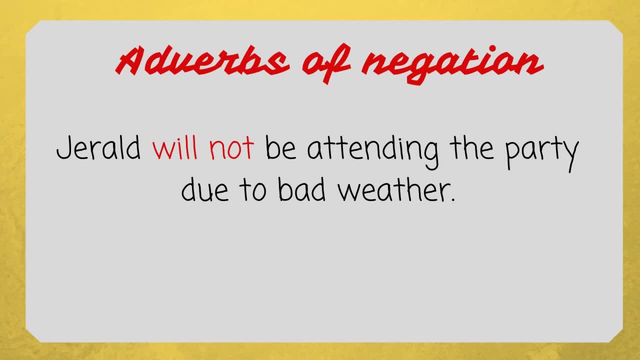 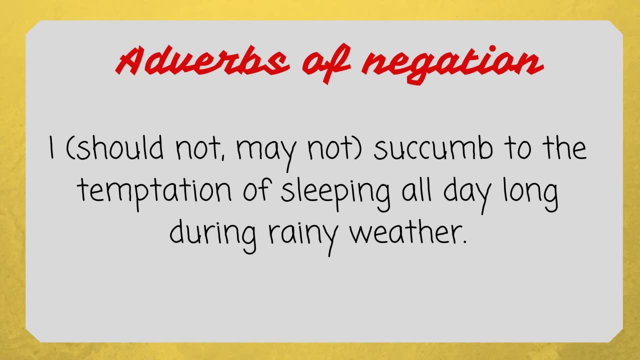 Okay, let's go to the next one. In this sentence, we will be choosing the accurate or the appropriate adverbs of negation that we should use in this sentence. Okay, I should not, may not, succumb to the temptation of sleeping all day long during rainy weather.